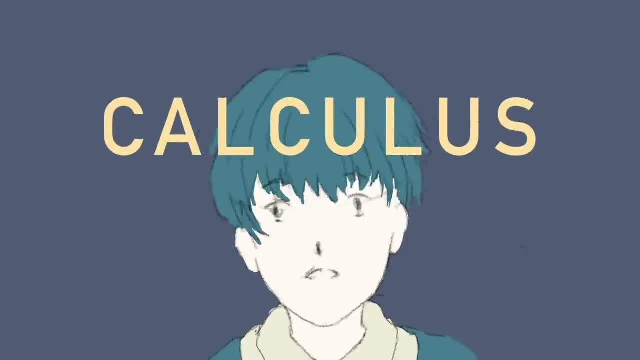 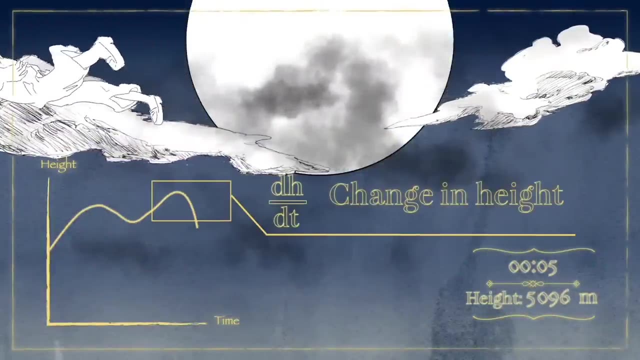 physicist Richard Feynman as the language of God, calculus. Scary huh. Well, it's basically just a description of changes in our ever-changing universe. Normally, when we talk about changes in stuff, we talk about the difference in the amount of stuff after the change. Well, we can also talk. 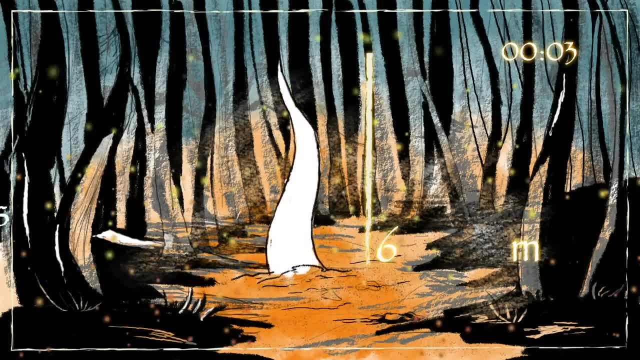 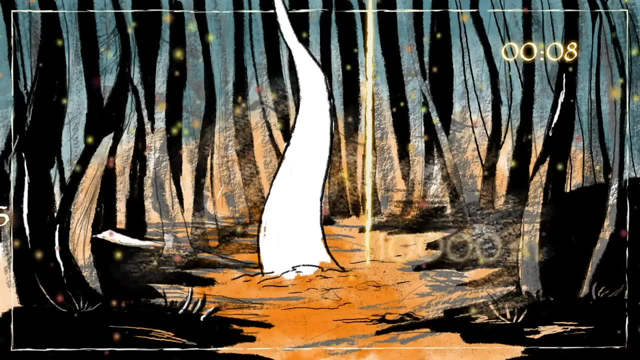 about how fast something changes, the rate of change, how much something changes in a period of time. To find the rate of change of the height of this bean sprout, we found out how much it has grown within the period of time. Dividing the height by the time gives you the rate of change. 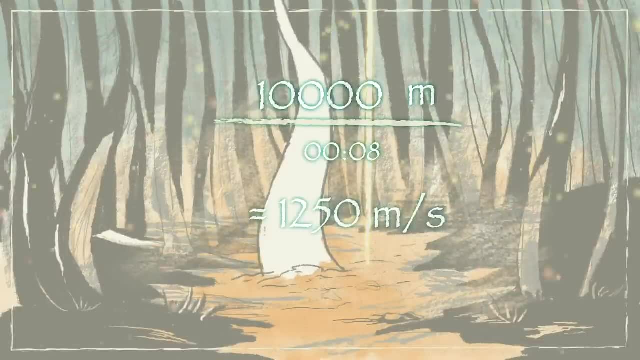 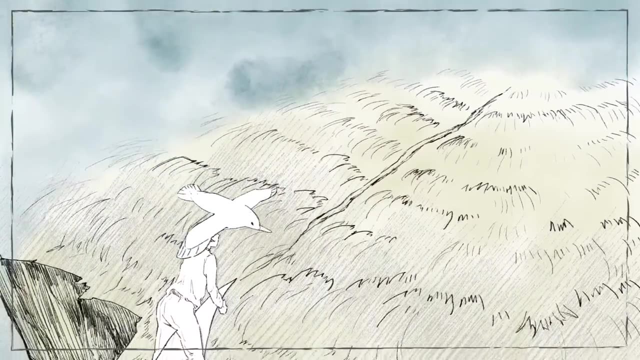 1250 meters per second, Easy right. But if you're a good observer you'll probably notice that most things don't change at a constant rate. So the method I just mentioned doesn't really indicate the variations in the rate of change. 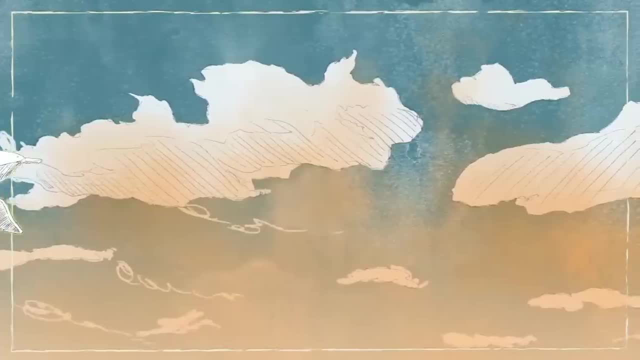 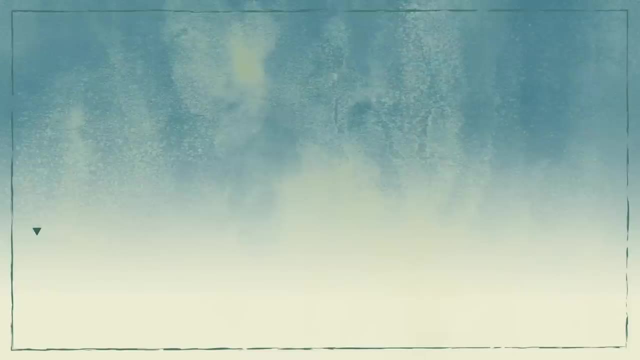 throughout the entire motion. Perhaps we can chop the motion up according to its speed, like fast period and slow period. Yeah, but it's perhaps still not precise enough. How about dividing it into smaller chunks, like tracking the change in the distance every second? 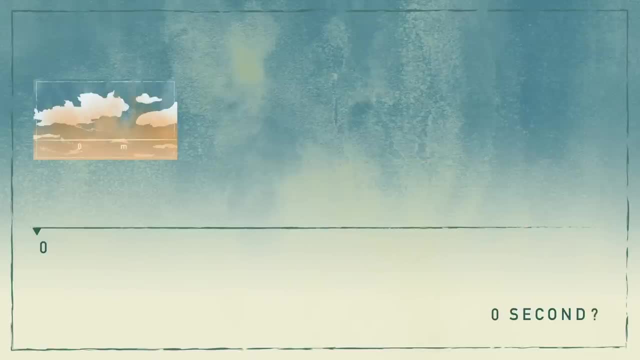 millisecond, nanosecond or even zero seconds. Wait what? Nothing can change within zero seconds, when time doesn't even pass Well, even a powerful subject like math can't change the rate of change every second, millisecond, nanosecond or even zero seconds. 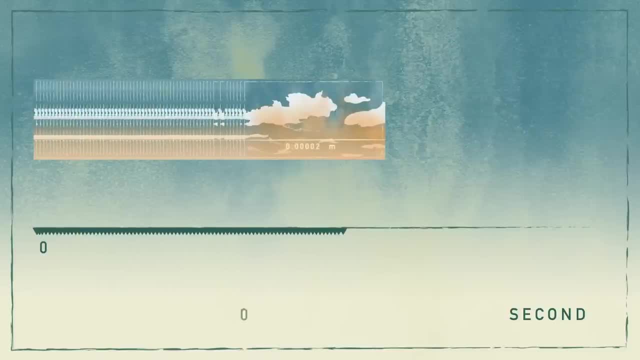 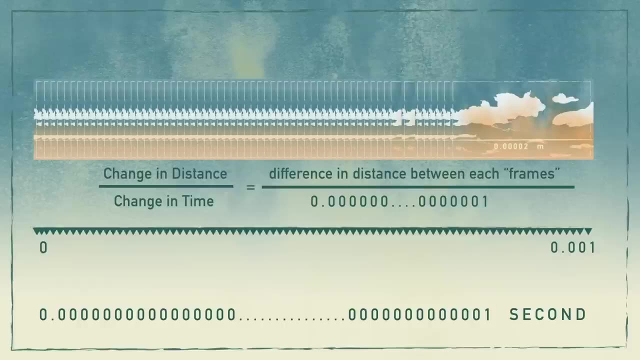 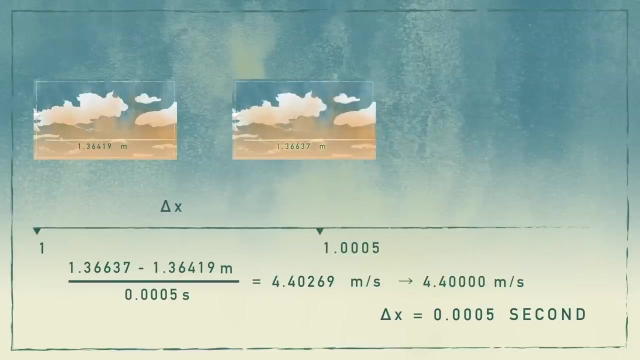 What we can do is to record the change within an infinitely small period of time- almost zero seconds, but not exactly zero. We call this small period of time delta x. As delta x decreases, you see the rate of change approaching a certain value. 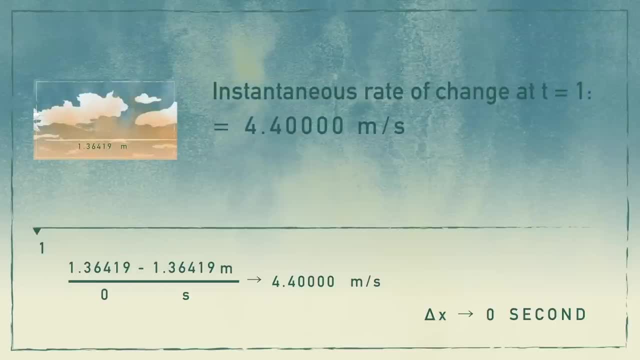 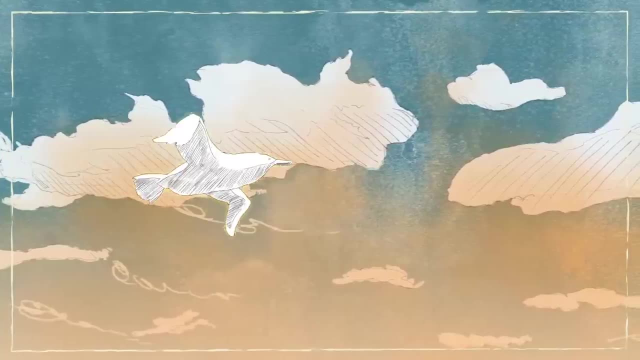 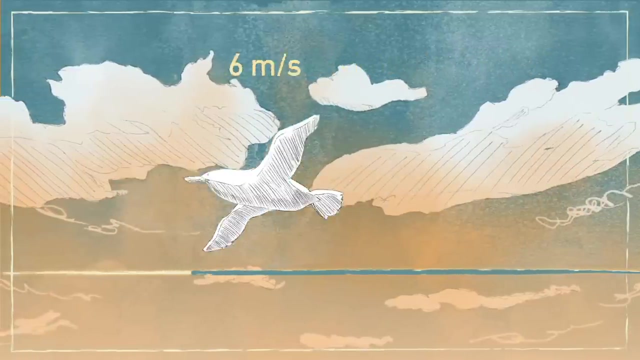 And from there we can approximate the rate of change at a specific moment. This process is called differentiation. What's so amazing about calculus is that not only we can use it to find out the instantaneous rate of change, but also to do the reverse, Given how quickly something changes. 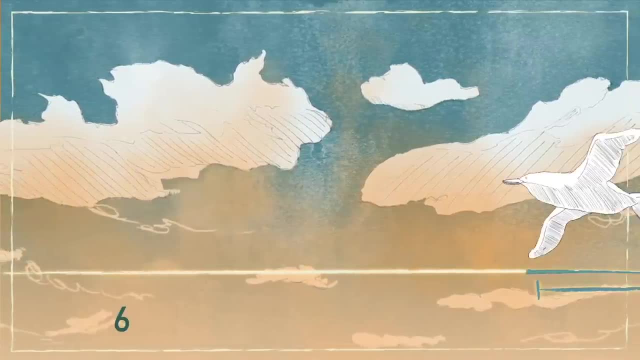 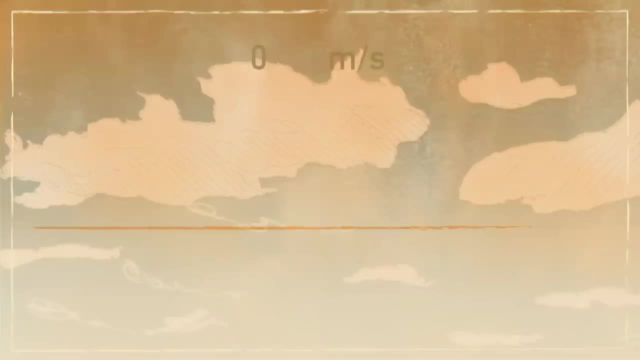 we can know how much something has changed. To find out the distance traveled from the speed, we can multiply its speed and the change in time. But what if the speed is not constant? Well, we can chop its motion up into very small periods, delta x, And then add all the distances. 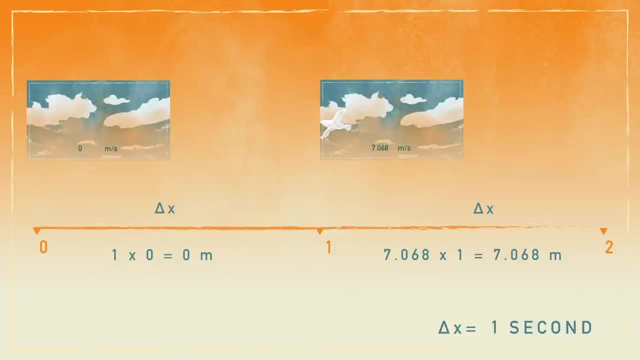 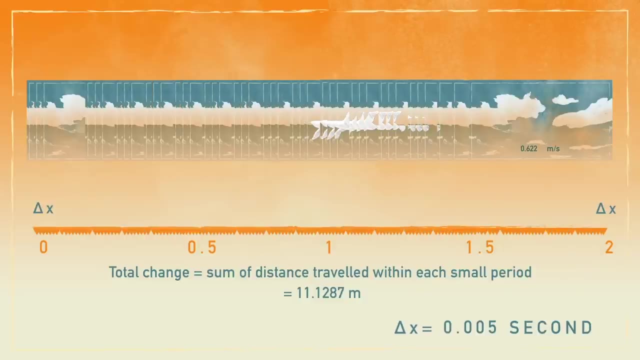 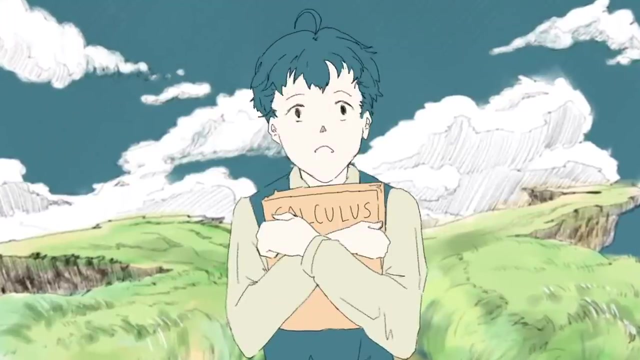 traveled within each small period up to get the total change in the distance throughout the motion. As delta x decreases is approaching zero, you can see the total change in distance approaching a certain value. This process is called integration. You might ask why do we care about calculus, apart from nailing exams? 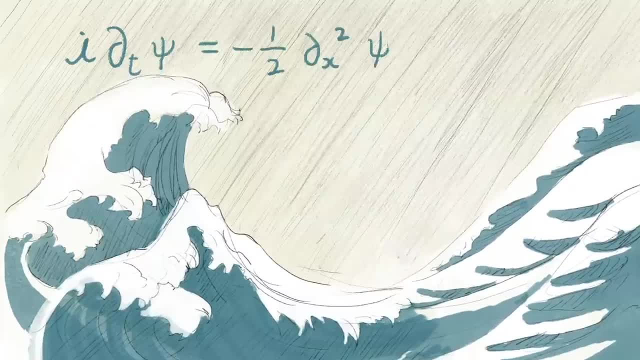 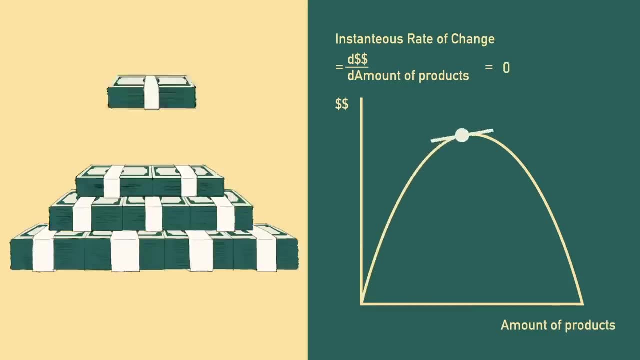 Well, many people do care. Scientists use it to describe the changes in our natural world, engineers use it to optimize their designs and economists use it to optimize profits, Even if there isn't any point in your life that you'll have to apply calculus to real 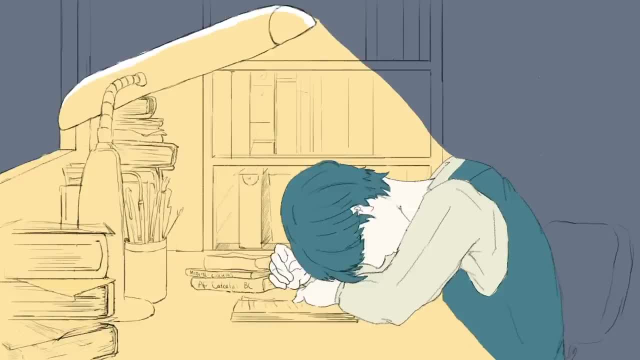 life problems. well, isn't the ability to see the world in another language pretty amazing? 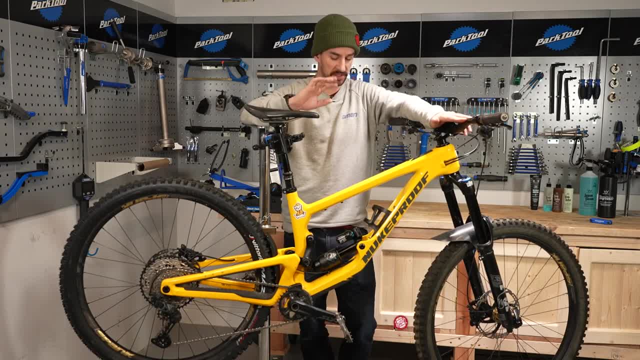 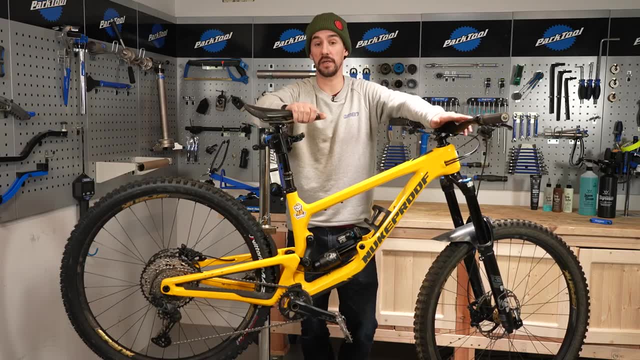 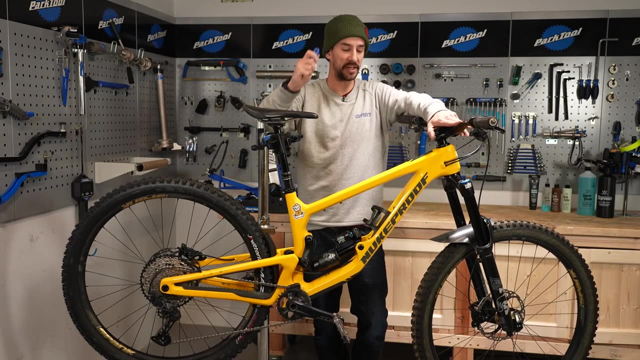 Thinking about a few things and doing a couple of essential maintenance bits is going to help your bike run nice and smoothly, but also keep your pride and joy lasting you a bit longer, hopefully. Step number one in making your bike last a bit longer is actually to do a regular. 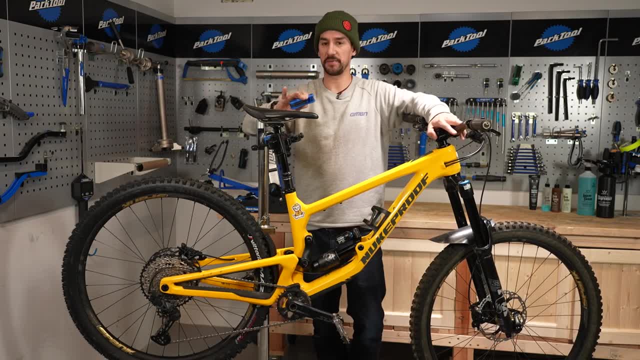 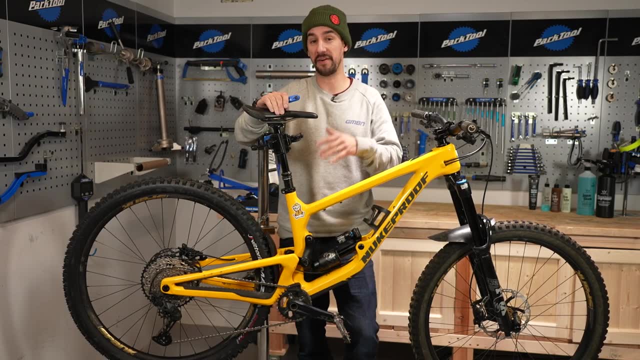 bolt check Sounds crazy, but I've done this myself and seen it happen quite a few times, where, if you don't keep on top of this, things can come a bit loose and it can start wearing your bike out or even damaging them. I've seen rear axles come out on a ride before and that completely smashes. 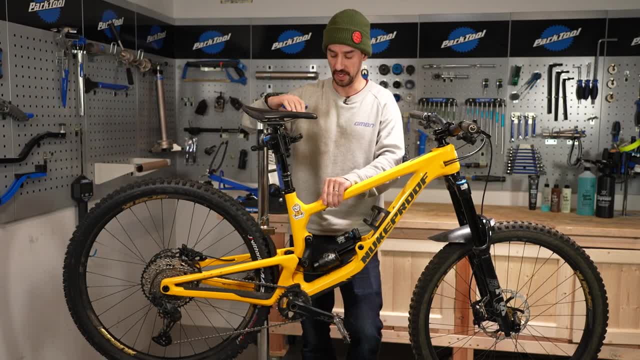 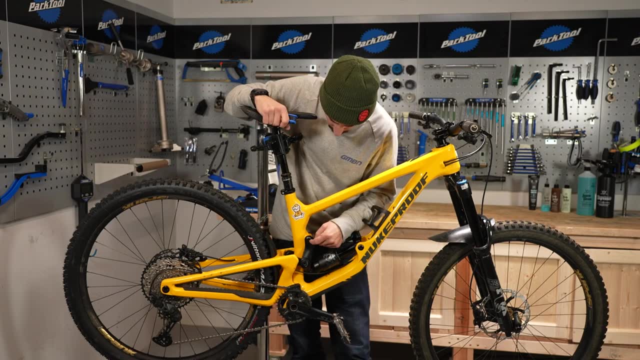 the back end of the bike. It snaps the mech off. It can do loads of damage. It's really important just to fairly regularly have a look at your bike. Sometimes I see one of your linkage bolts- your pivot bolts- might have backed off a bit and you can see a little gap. Obviously that means 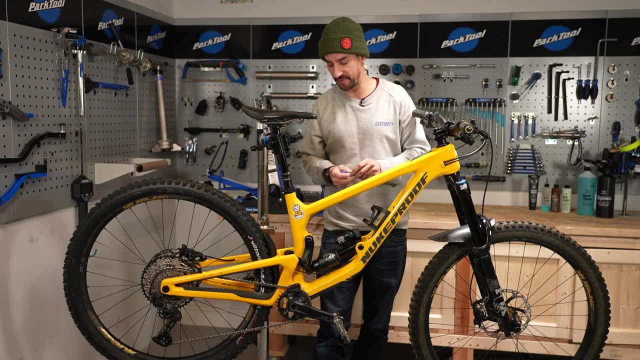 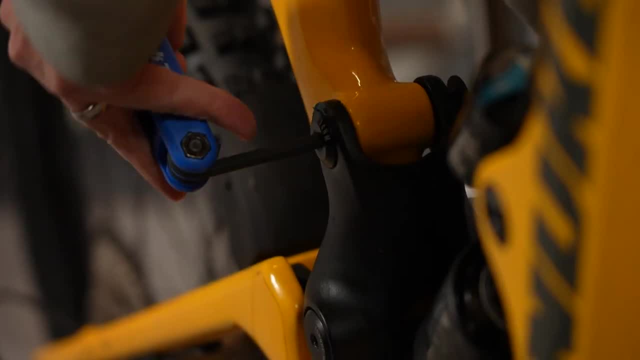 I haven't checked it often enough, but hopefully after a while you'll get a bit of a feel for what's coming loose in your bike, If actually something might need a bit of loctite, particularly on pivot bearings on full-spension bikes. I've done that quite a few times where